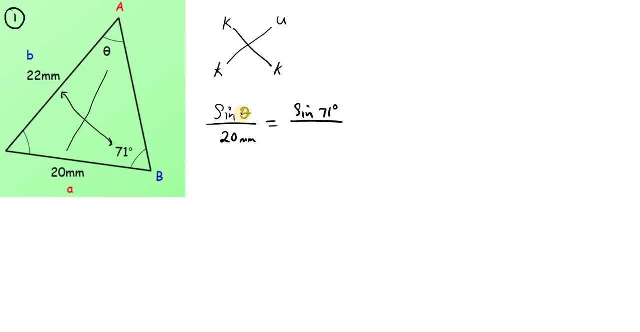 going to be sine. Now, please note that we have angle above the division line, In other words angle in the numerator for this fraction. So for this fraction we should also have angle in the numerator And remember, once you have an angle you should have sine next to that angle known or? 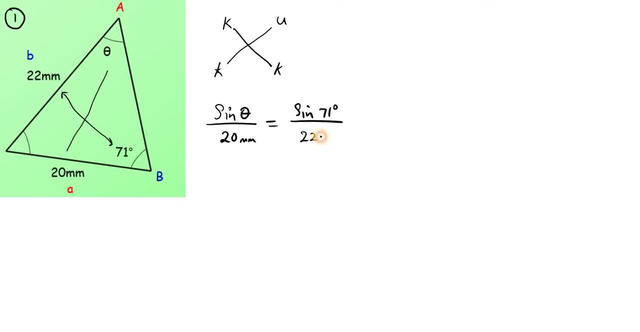 we have 22 millimeters. so now, once we have this situation, we can now proceed to find angle theta. to find theta, we're gonna remove the 21st, so the 20 is in the denominator, in other words, it's dividing sine theta. so once transposed, 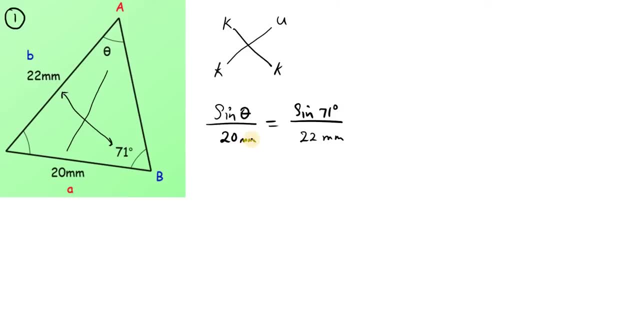 it will move from division to multiplication and once it multiplies, therefore, it moves from the denominator to the numerator. so we'll have sine theta equals and, as I said, 20 move from the denominator in this side of the equation to the numerator in the other side of the equation. so we have 20 sine. 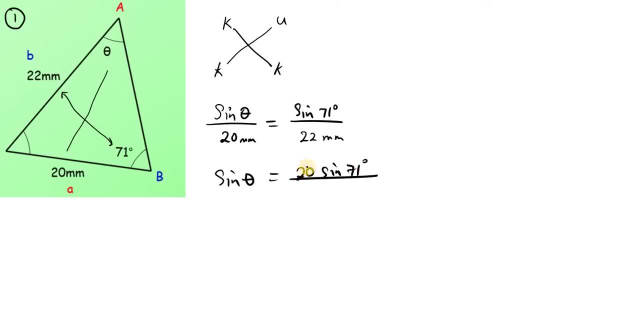 71 degrees. it's 20 years, 21, 20 millimeters multiplied by sine 71 degrees. but I'm gonna leave off the units for now. now I'm gonna put back the 22 millimeters, 22. then I want to find theta, remember, that's the goal. so when, when I 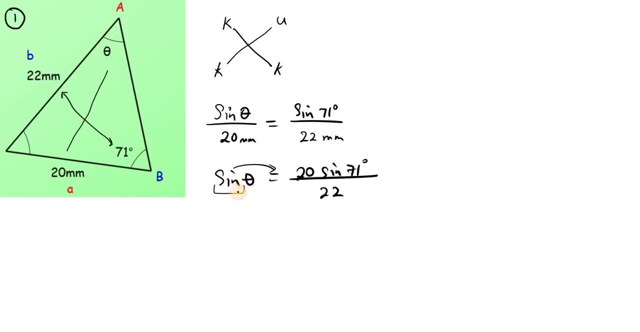 transpose sine by itself. notice, I'm moving sine by itself, not with theta, but just by itself. once that's the case, we're gonna use sine inverse, so sine inverse of 20 sine 71 over 22. so you put that in your calculator. all right, don't? 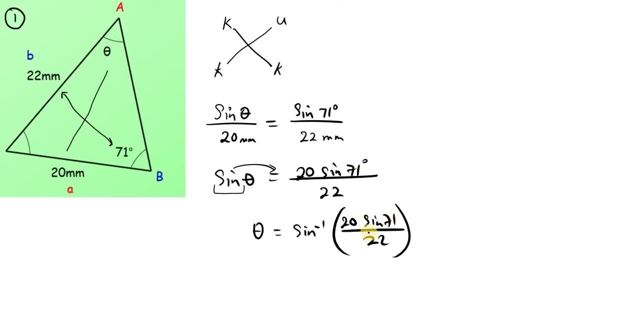 put the degree symbol in your calculator, of course, not just put this that you're seeing here in the calculator. you may have to put the 70 one in brackets, so open bracket. then you can click on the ABC button or, if you have a button like this, a fraction button. once you insert that then in this: 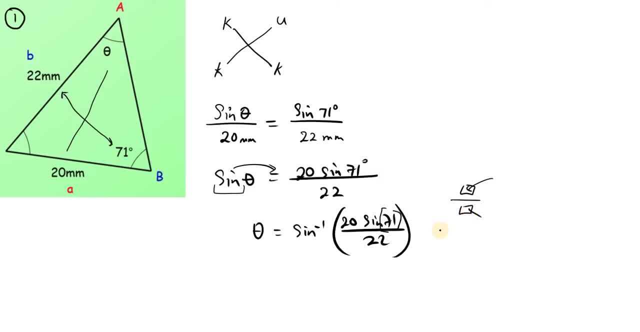 the numerator you'll put the 20 sine 71 and in the denominator here you'll put the 22, close bracket. all right now to get sine inverse. of course this part is very essential. to get sine inverse, you'll need what to press the shift key. 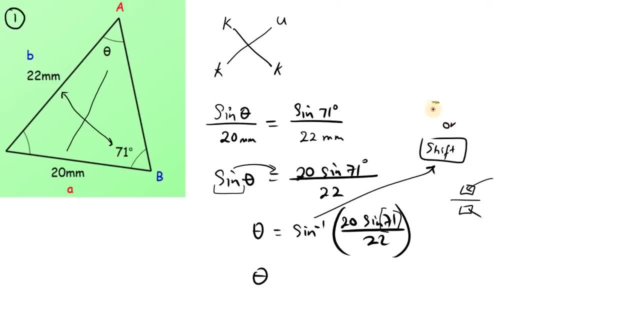 you may not have a shift key in your calculator. it could be this key that says second function. so either one of these, and then you press sine, your calculator will display what your calculator will display: sine inverse. as a result, open bracket. and so here you will enter the information 20. 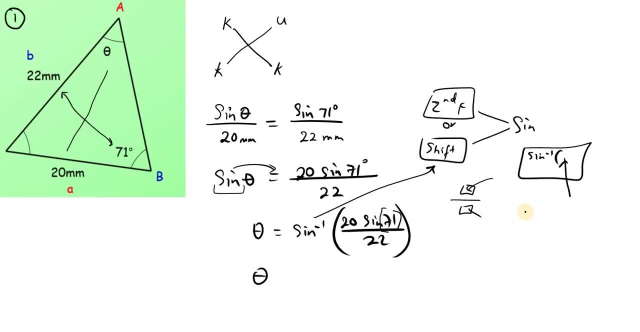 sine 71 divided by so careful when you're entering this. so you say 20 sine open bracket 71, close bracket, then put division and then press 22, then of course you close bracket. remember you want to close this bracket when you're done and you should get what value point two, six, seven, four, seven, eight, zero, eight. 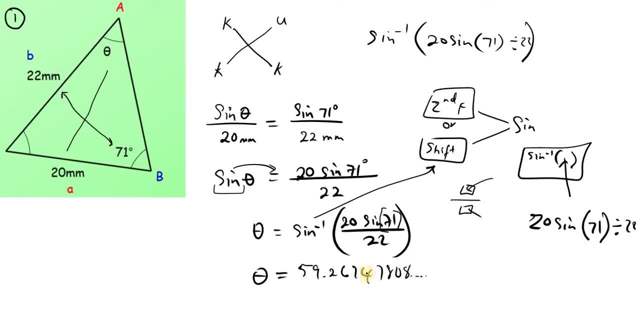 all right, that's what's displaying on the calculator. I'm sure they have more digits, but this is what my calculator can hold. so theta, the, the unknown angle here that I'm trying to find, let's say to three significant figures. the first non zero digit is my first significant, so that's five my 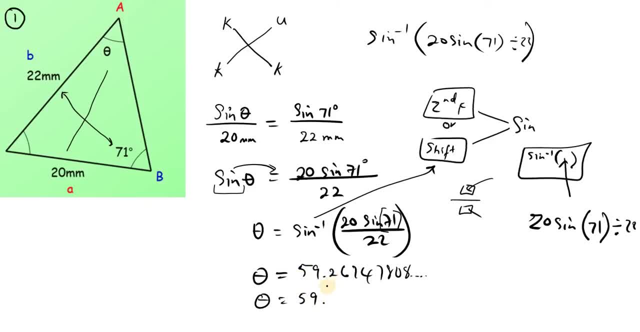 second significant figure and the third one which is the last of the significant figures I want, I would have to check the next digit. this next digit is six, falls in the category of five or more, so I'll add one to this two. that would be three, so it's fifty nine point three degrees, remember I will should be in degrees. 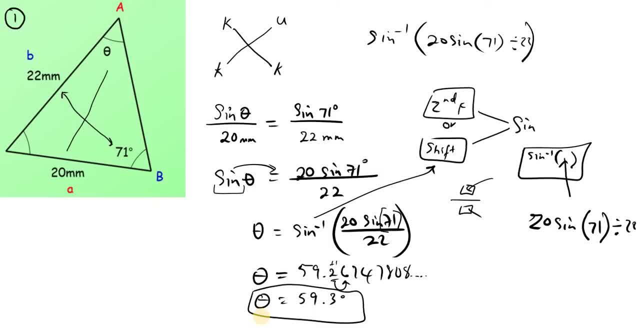 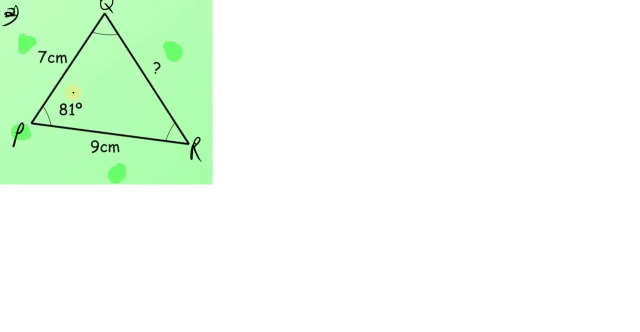 that's that, okay. so hopefully that was helpful. now let us move into another question. let's look at this one. so we have this triangle P QR now. once we have angle P here, I will label this side as comma letter P. once I have angle Q, here the 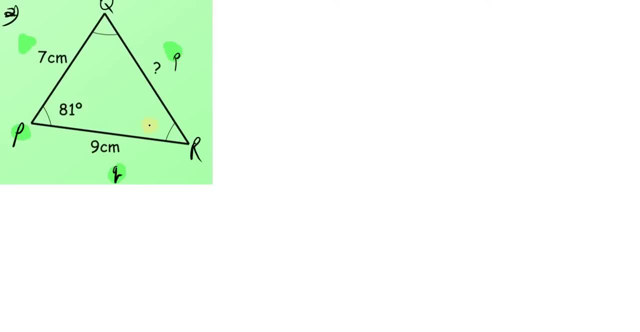 side that faces it, I'll label it as comma letter Q, and once we have angle R, the side that faces it, a small common letter R. okay, so now I need to decide on which side to choose. am i going to use a sine rule? still, can i get an x out of it? well, let's check. do we have now? if you? 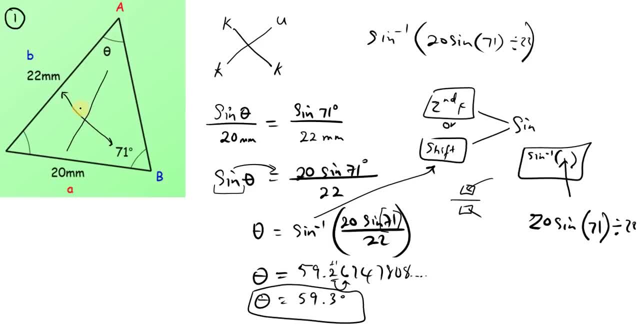 go back to the origin. the first question. did you notice that we have for this line here? we have a angle at one end and the side, the measure of the side on the other end, the known angle on one end, the known side of the other. so no known. so that's a full pair. for the other line we have a half pair. 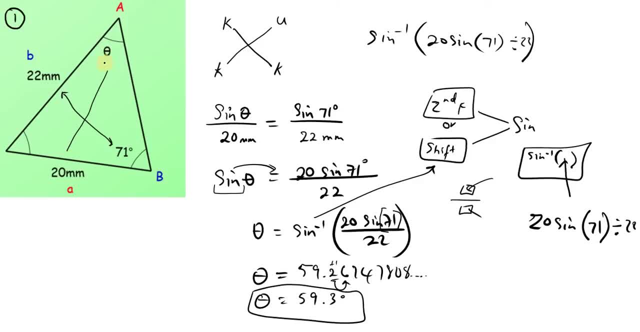 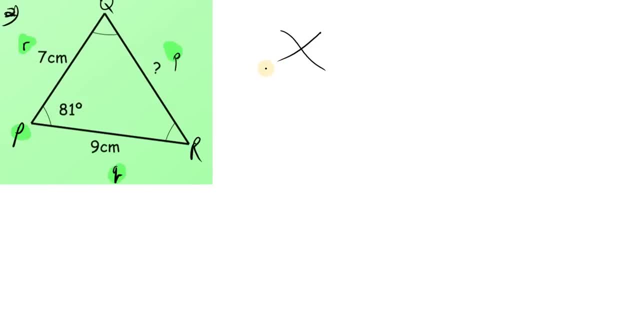 in other words, the. the side is known, as in this, but the angle is unknown. so we use sine rule in this case. now let's go to this one. do we have the same same scenario here? well, if you look at this, if you look at this, we have a known side, but an unknown angle. if you look at here: 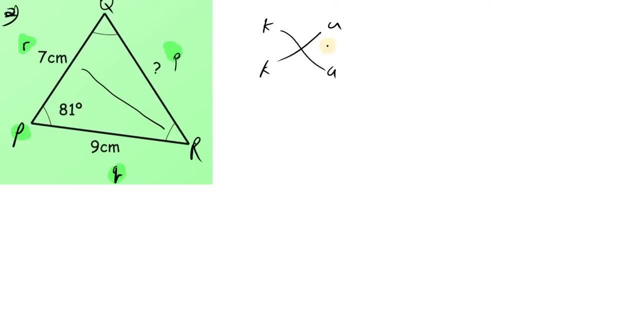 we have a known angle but an unknown side, so we can't use the sine rule. so we can't use the sine rule. for sine rule we need to have a full pair. we have a half pair here, in other words, we have an unknown. we have a half pair here, in other words, we have an. 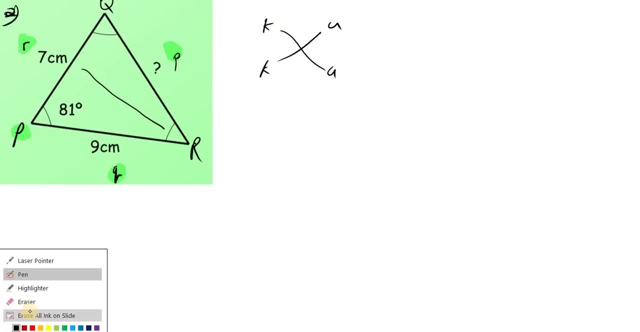 unknown. so we cannot use a sine rule. but we have another rule that we may want to consider, and that rule is the cosine rule. now for the cosine rule. for the cosine rule, we have this formula: a squared is equal to B squared plus C squared minus 2 times the product of B and C times cosine of the angle. a notice: 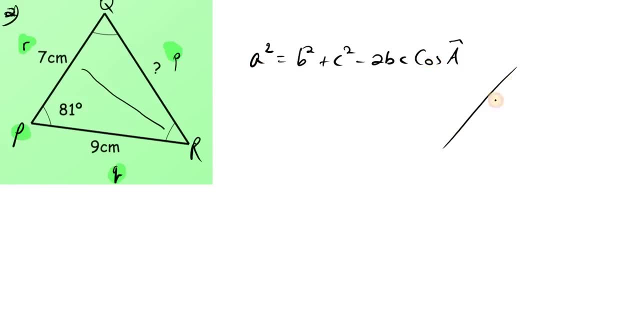 that we have comma letter a here and capital letter here. well, this is the situation. so let's say we have the triangle ABC. all right, triangle ABC. now. this is angle a and it faces what side little a we have. angle C and it faces what side little C we have. 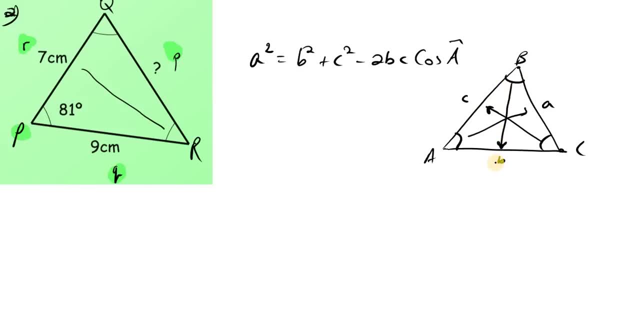 angle B and it faces: what side? little B. so when I talk about side AC, I can say side B. notice that when I say side AC, I did not mention B, so that's little B, so we can use B to represent ABC. when I say side a B, I didn't mention C, so we can. 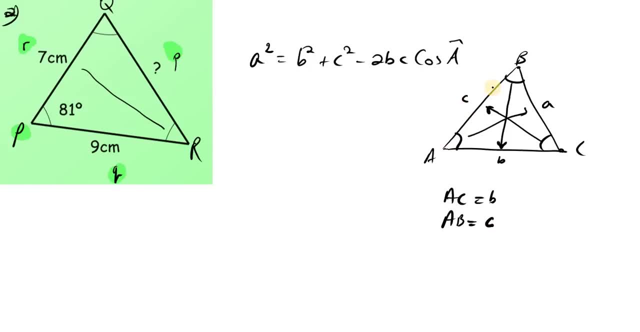 use comma letter C, as we can see here it's come. a letter C represents a, B. I want to say BC. notice I didn't mention a, so this side BC. I can actually use a to reference that side. but again, you can dare, you can actually see that opposite side a is angle A, so we can see side faces, the. 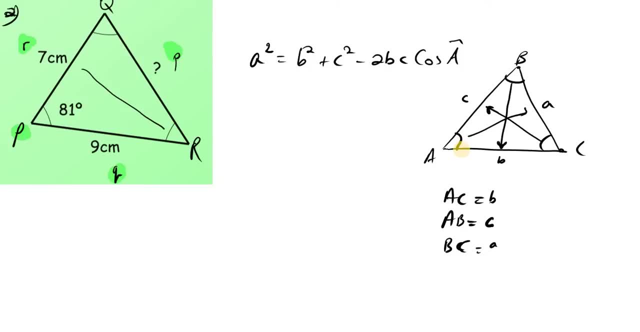 angle with the same letter. just one is common, one is capital. okay, so if you notice in the, in this cosine rule formula, in this cosine rule formula, what do we have? we have a case where we have side a facing what angle a, and that's how it always is. whatever letter you have here, you would have the same letter for the. 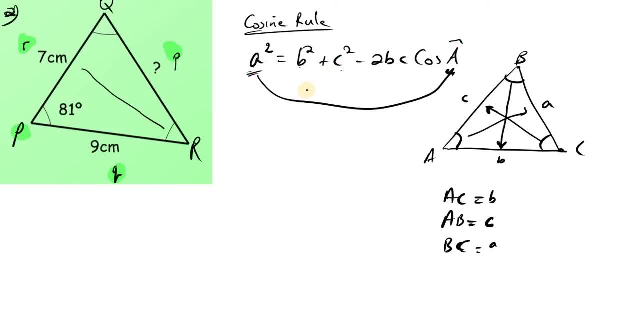 angle. now these are the sides. a, b and c are the sides. b is the side of the triangle. c is the side of the triangle because there are common letters. right, common letters are used for the sides of the triangle. we have b and c here again now. this b is the same as this b, same measure. this c is the. 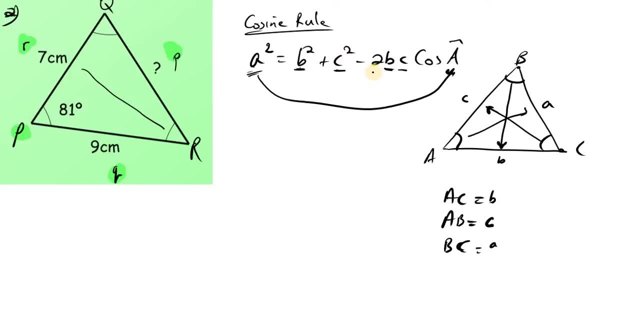 same as this, c, same measure, right referring to the same side. okay, so now you get that. now i also want to mention this right. i want to mention that you see these, these two sides, b and c, again repeated here, those two sides are the sides that form the angle that comes right out the cosine. 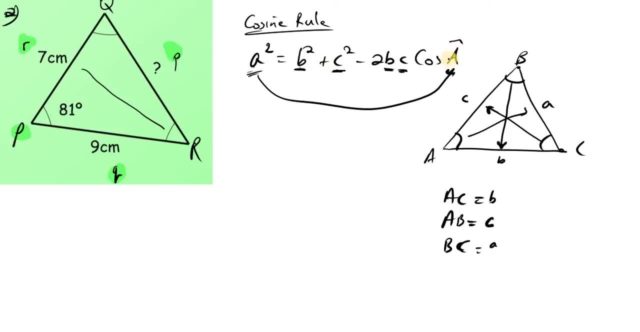 here. so b and c form angle a. let's look at this triangle here. do you notice that we have sides what? let's use a different color. let's look at this. we have side what, b and side c. let's look at it. this is side b, this is side c. 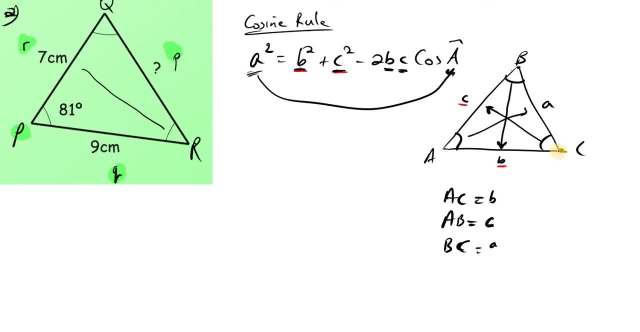 C and you notice that sides B, which is this side here, and side C, which is this side here, they actually do what they actually form the angle here, which is actually angle a. so size B and C are the two sides that form the included angle. okay, so we have B and C forming angle a, which is this angle right there, so that 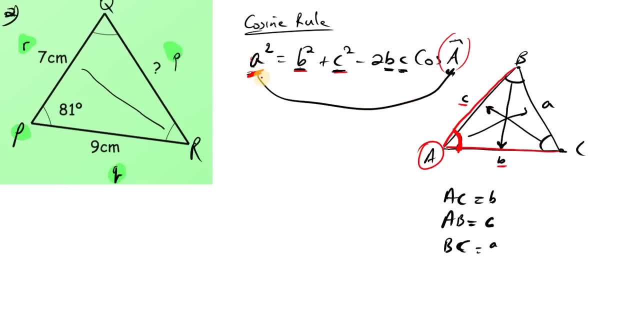 we want to keep that in mind. and what about a here we didn't mention a. well, a is a side, that is what opposite inside, that is opposite the angle a. so, if you look at this opposite, this angle a, here is what the side a. all right, so let me. 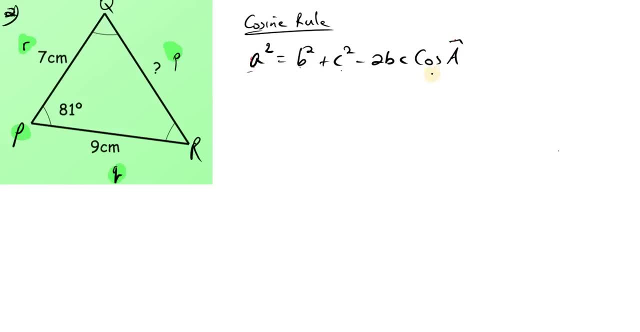 just clear this well. we said that this is the angle that faces a particular side a, facing what side a and angle a is formed by the two sides. B and C got it. so these two sides- B and C- form angle a, B and C. B and C form angle a and opposite. 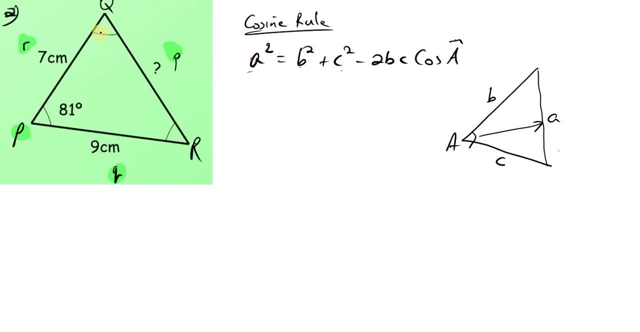 angle a is side a that we have here. now, when you look at this triangle here, what are you seeing? you're seeing these two sides that form this angle. ox. 해서 dois lados será a Ara, B e C but a Miguel". these two sides would be our B and RC, the, the two sides that form the included. 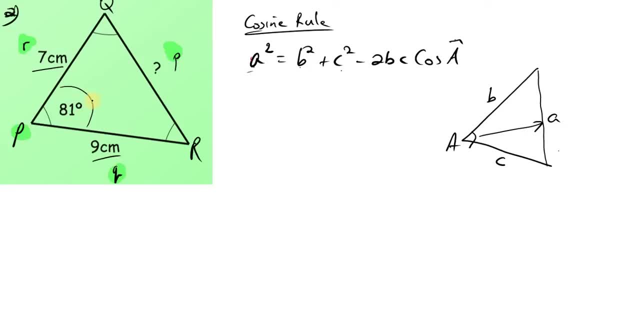 angle and opposite, the included angle is this side: ox, então acosta como cartão incluido. in relation to this formula, we may not be given the same letters, but we should understand what these letters are: ill bananas presenting. so again, B and C represent the two sides at form angle a. what you 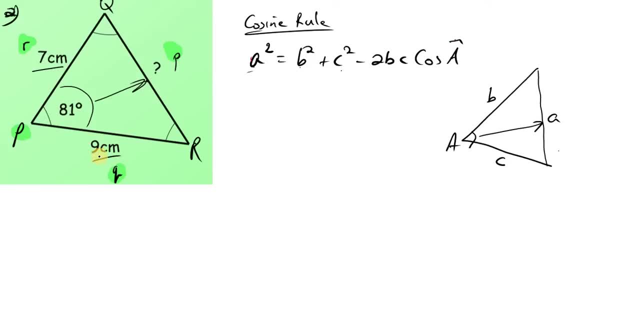 sides form. sorry, well Panorama, when you're looking at 62 inches ぐらい ros, in this case q and r, the seven centimeters these two sides, r and q, form angle p that we have here. so the side that faces this angle is little p, so that's what we'll put here: little p that faces. 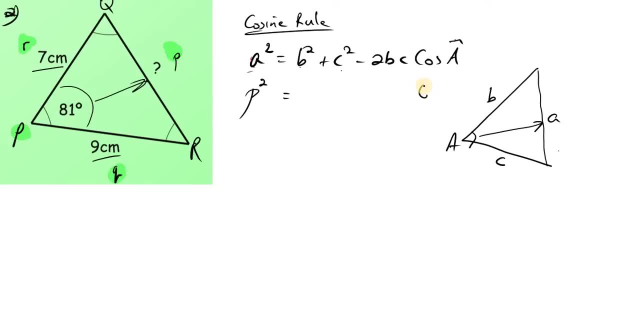 the angle. so we square it and at the end we have cosine of the angle that faces p, just like we have here the angle that the side that faces angle a is side a, the side that faces angle p side p. so what we'll have here is capital p for the angle that faces side p, and b and c being the side that. 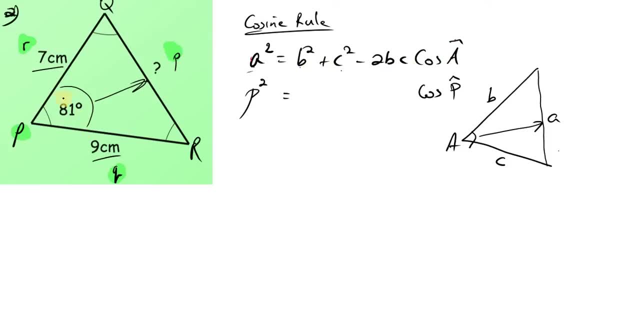 form angle a. so the side that form angle p is side r and q. so we'll have r squared plus q, squared minus two times again br and q times cosine p. so put that into perspective. we have p squared equals r being seven, seven squared q being what, q being nine, nine. so we put the nine squared minus two times the product of 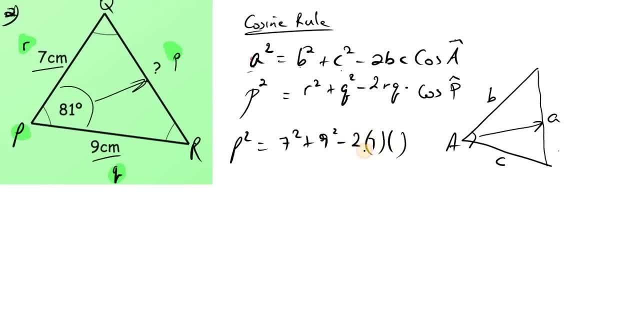 r and q, so r being seven. so whatever number we have here, put it here. whatever number we have here being nine, put it here. cosine of angle p being 81 degrees. okay, okay, now let's just take this out, just so it doesn't confuse us all, right? so 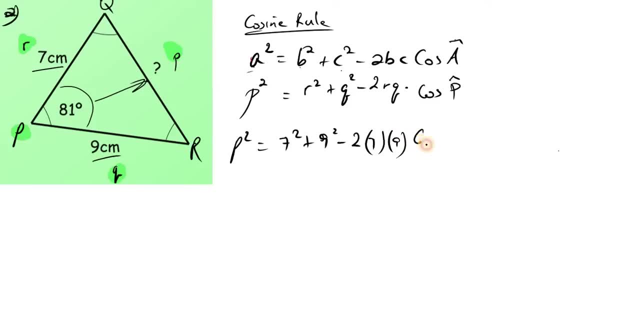 so this could be cosine of the angle, which is 81 degrees. so we have p. squared is equal to now. what you can do here, you can just plug this entire expression in your calculator. if you have a double display calculator, you can put it in. if not, then you can just break it down seven squared. 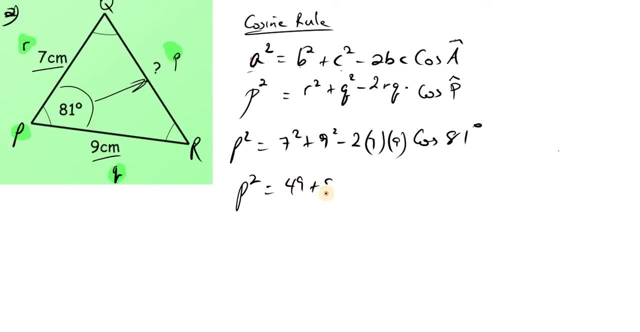 is 49, eight squared is 81, and then we can see: two times, seven times nine. can put it in a calculator: we get one 26 multiplied by the cosine of 81. so cosine 81. no inverse here, because you just straight cosine and we end up with: 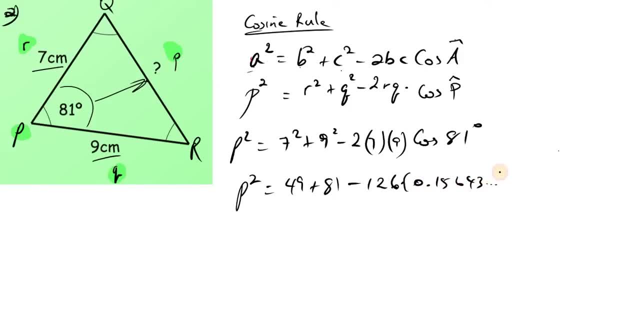 0.15643, etc. right now, again, Again. you want to ensure that you multiply these guys, And so you're working out these two parts separately, right? So P squared is equal to what: 49 plus 81.. That gives us 130.. 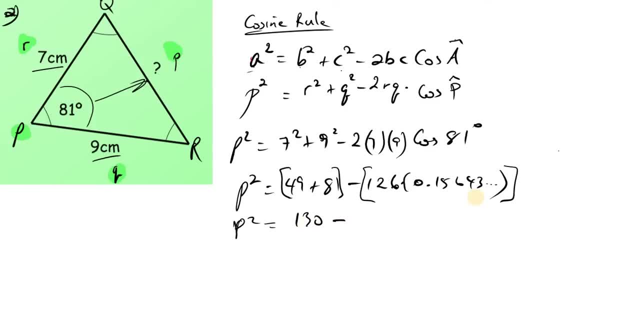 Always do multiplication together before you add or subtract. So that's 126 times cosine 81.. Or you can just say 0 point whatever. But I can just multiply this part in my calculator 2 times 7 times, 9 times cosine 81.. 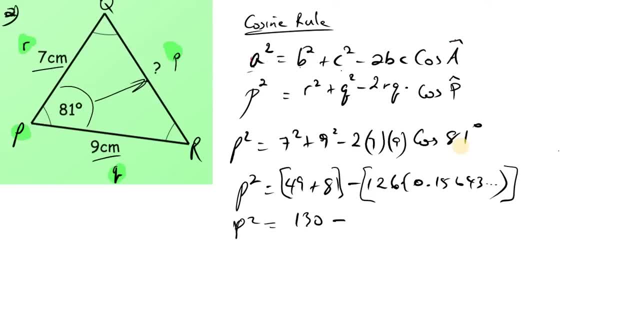 I think that will give us a little bit more accuracy than writing down everything. So 126 times cosine 81.. That gives me 19.7107426, etc. But if I want to write up to three decimal places, it's always good to use up to three decimal places. 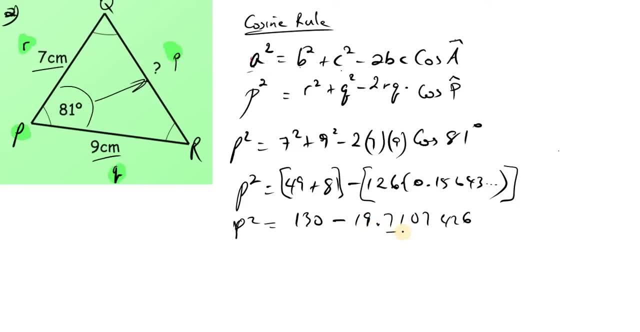 Before the final answer: So that's 19 point And I'm going to write the 7.. That's first, second and third decimal place, So I'm going to chop everything off. Then I've checked the next digit. This 7 falls in category 5 or more. 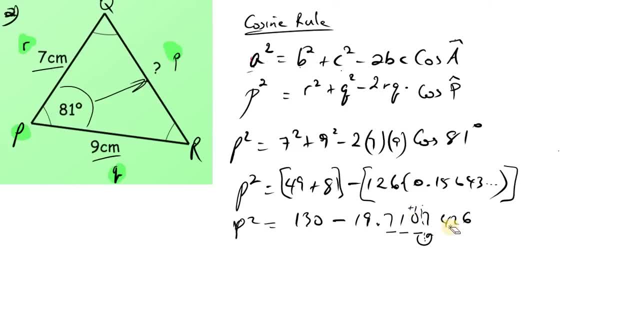 So I'll add one here, And so my answer is just going to be taking all this off: A 1. Replacing that 0.. Alright, so now I'm going to have: P equals the square root of Now. I need to work out this portion here. 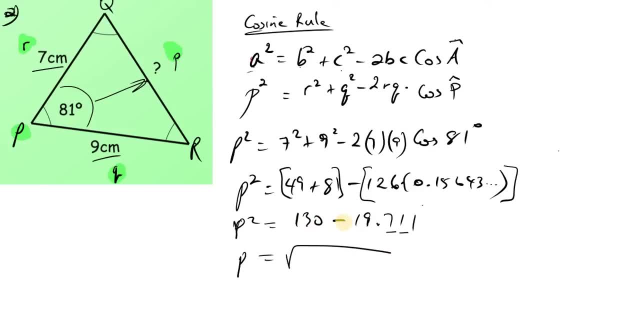 What is 130 minus 19.711?? That's 110.289.. Now you might be wondering: okay, how did I get a square root there? So let's go back to this. Let's go back a little bit. So I put back this P squared and I work out this portion. 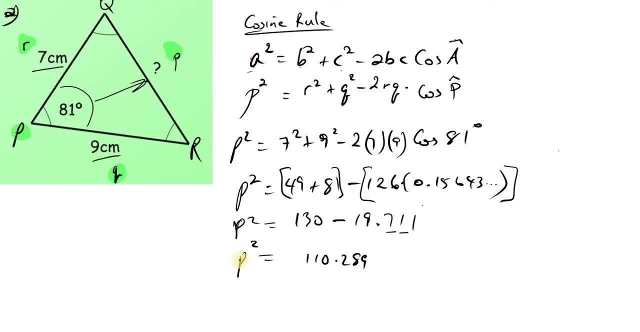 which gives me this up to three decimal places. To find P, I need to remove the square. To move the square, I want to transpose it. The other side becomes the square root. If not, if you don't understand that, then I can say I square root the square. 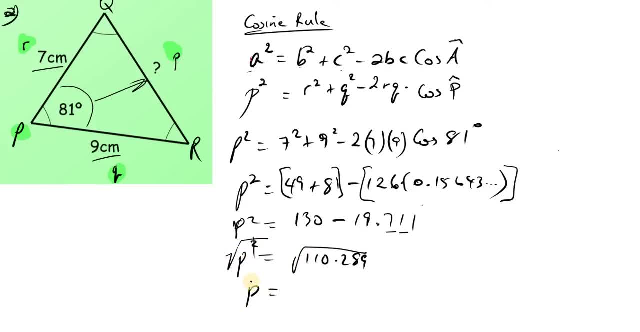 Take it off. So I square root the side as well. So technically it's like you transfer the square over a square root And the square root of that 110.289 will give us what. So I press square root and I press answer that I have originally. 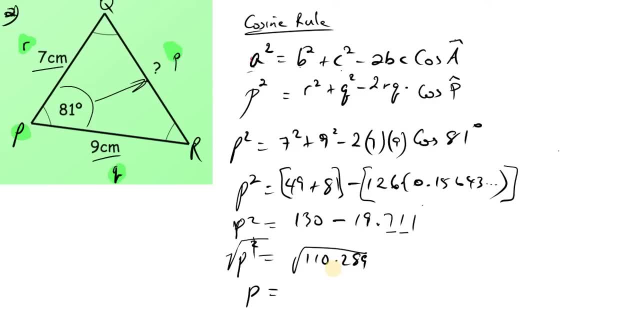 which is the 110.289.. And I get 10.5.. That's up to three significant figure, that's be 10.5.. Okay, I have 0.1, 8,, blah, blah, blah. So technically it's 10, point. that's the first. significant is one. 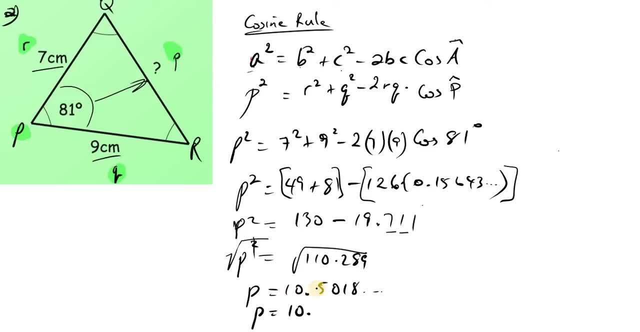 Zero is significant because it's between two non-zero digits, And all non-zero digits are significant, But because this zero is in between, the non-zero digit is significant as well. So that's one- two. This is my third significant figure. 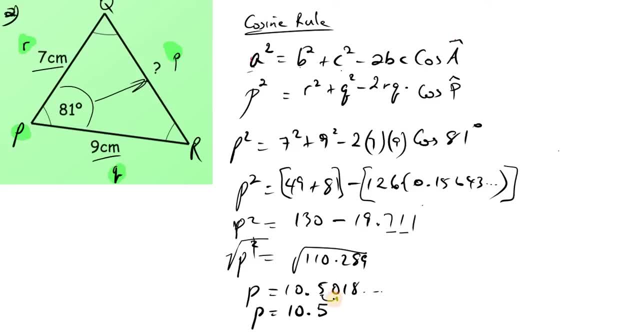 Why didn't I add one to it? Because the next digit is less than five. So again that's 10.5.. So again it's chopping them all off. And since we're looking at side P being the side of the shape, the triangle, 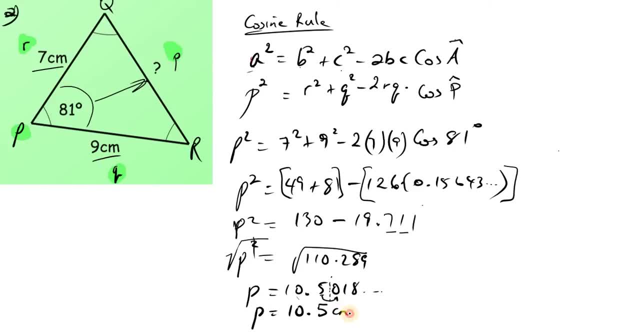 and we're dealing with centimeters, then this is actually 10.5 centimeters. So this is the length of the side I'm looking for. All right, hopefully that was helpful. So notice that I didn't just show you the formula and just plug in the values. 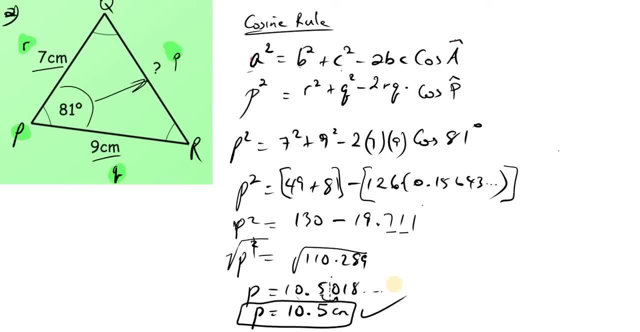 I also want you to understand what these letters or variables represent. And again, just in summary, just so you remember, in the formula, a squared equals b squared plus c squared minus two, b, c, cosine, a, the, what The b and the c represent, what 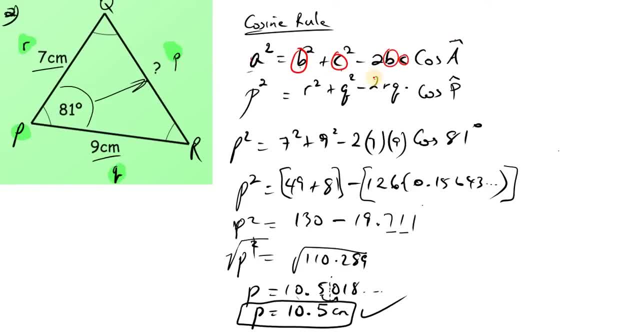 The b and the c, which is here again and here again. The b and the c represent the two sides that form the included angle right here of 81.. An included angle is our a, In this case, given as p. That's why we have p here. 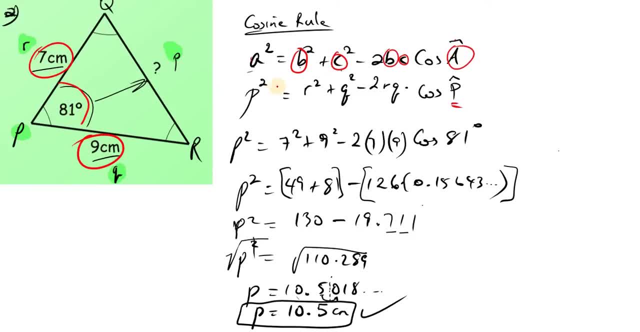 And the two sides actually form the included angle. Even though we say it's b and c, they are b and c's. They are b and c. sorry, then we actually have different letters in this case, So we use r and q to represent those. 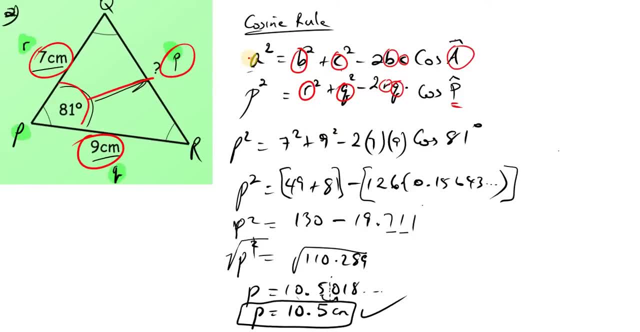 And obviously opposite this angle is our a, but in this case p. So in order to find p, we substitute from here all the way here with all the variables, plug them in our calculator. So we can actually plug all of this in our calculator and we should actually get this. 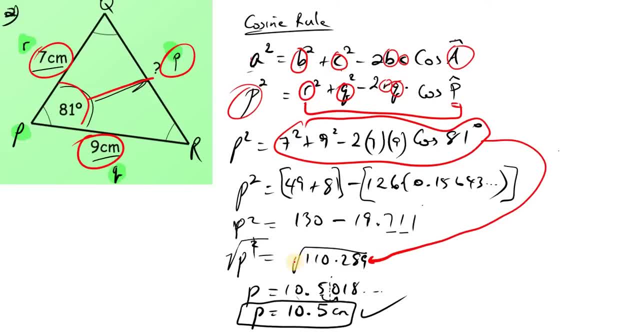 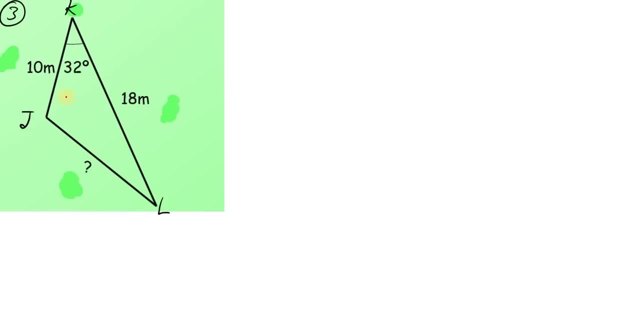 number below here. run it off to three decimal places, then find the square root of it. give us 10.5 to three significant figures. Okay, so now you understand that. Let's go to the next question. We have triangle j, kl and we want to find the angle here. 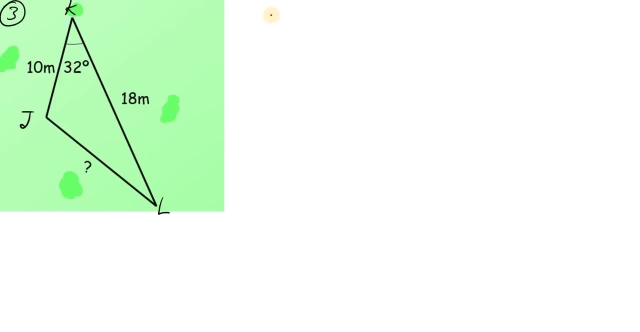 Can we use sine rule or cosine rule? Well, let's see if we have a full pair Again, at the end of this line we have known, known. So we should have a full pair. One end we should have a known, the other end we have unknown. 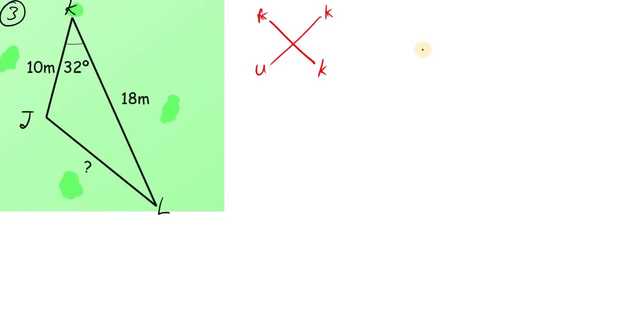 Doesn't matter which end, we have the known or unknown, Or even if it's like this, we could have the unknown here, known here, and the other side, the other line, we have known known, As long as on one side, one line, we have both knowns and the other we have one known and one unknown. 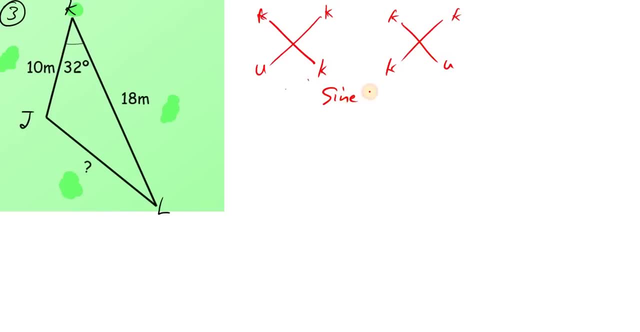 Then we use the what. Then in both cases we use a sine Rule, As we see with cosine rule. though we need three. we need all three sides of the triangle. Doesn't mean all three sides has to be known, but as long as we're dealing with three side and an, 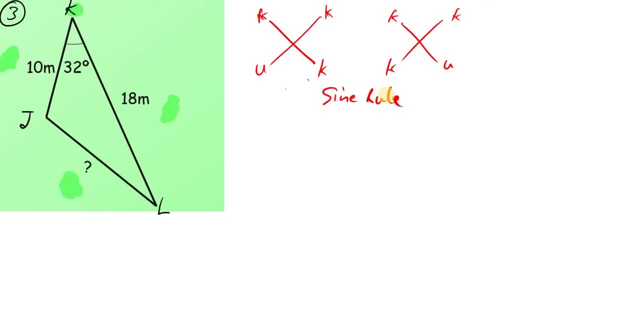 included angle, then we're good. So let's check this out. Do we have three sides dealing with? Okay, we have this side given, we have this side given and this side requested. So we have three sides that we're dealing with. 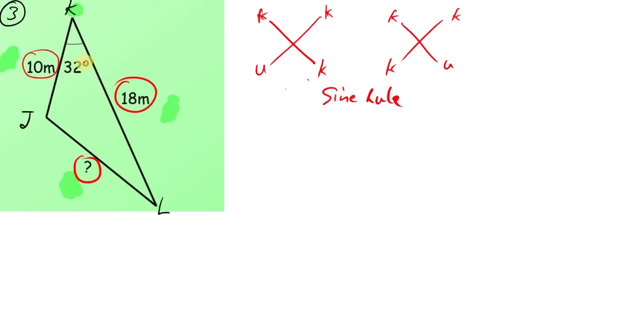 Two given, one requested. So that's three sides, right. And do we have the included angle? Yes, we have the included angle. So once we're dealing with three sides and the included angle, we use the cosine rule. Now for the three sides, two must be given or all three given. 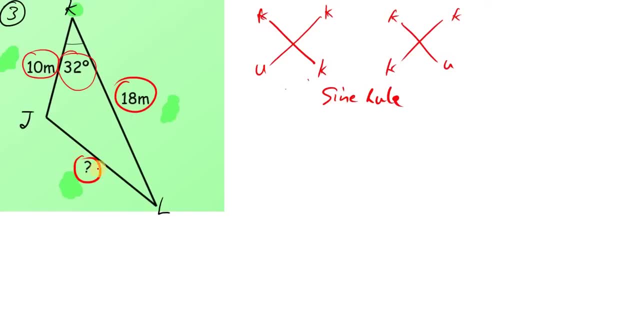 If only two sides are given, then we're asked to find the third side, but the included angle must be given. In a case where we're given all three sides, then the included angle must be requested. Okay, So therefore, we're not going to use the sine rule, we're going to use the cosine rule in this case. 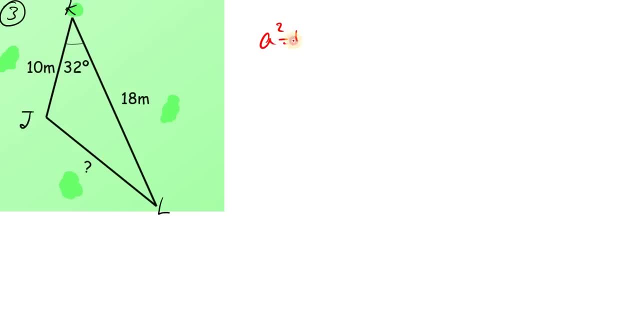 So let's look at it. So the cosine rule again is: a squared equals b squared plus c, squared minus 2bc. cosine of angle a. All right, Do we have the two sides, b and c, that actually form angle a? Let's look at it. 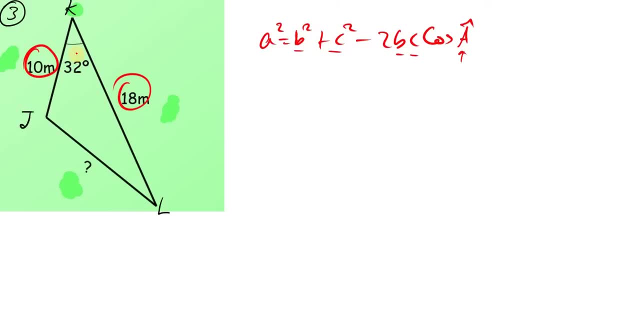 We have two sides of a triangle here and we have an angle in between both of these two sides. This angle is adjacent to both sides, So the included angle is given and the two sides that form the included angle are also given, But we are requested the side that faces the included angle. 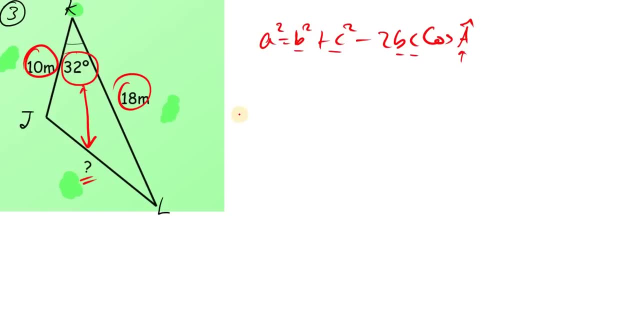 So cosine rule, Since we're asked to find a side, then a will be our side in this case. So we have a squared. In this case, a is really what. Since we have a capital K here, then this side is going to be common letter K. 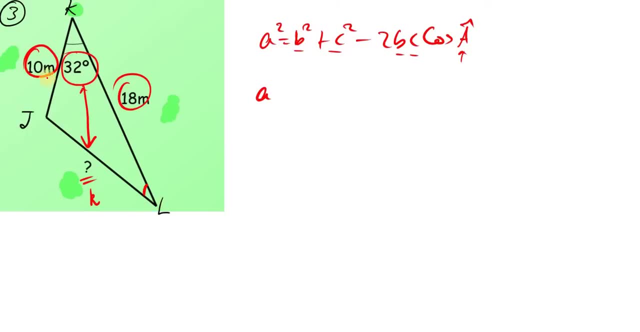 Okay, Since it's a capital letter L, then this side will be common letter L, And since the capital J that we have here, then the side that faces it will be common letter J. Okay, So we can actually use those letters instead of the original formula letters. 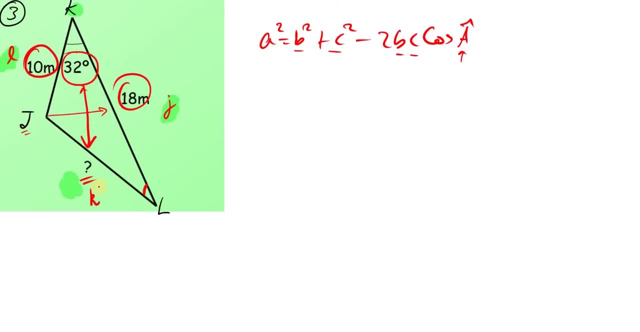 So our a is really what The side we're trying to find, which is going to be K, So we can see, we can actually say K squared is equal to the two sides of a triangle. Okay, Okay, Okay, Okay. 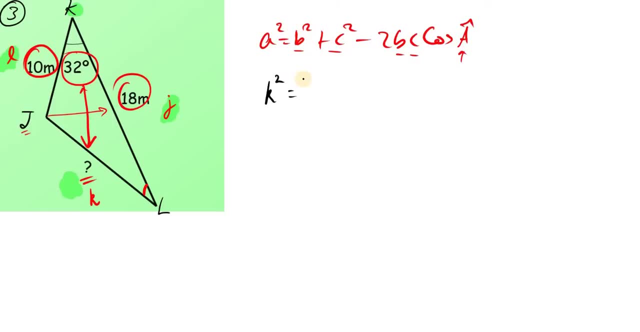 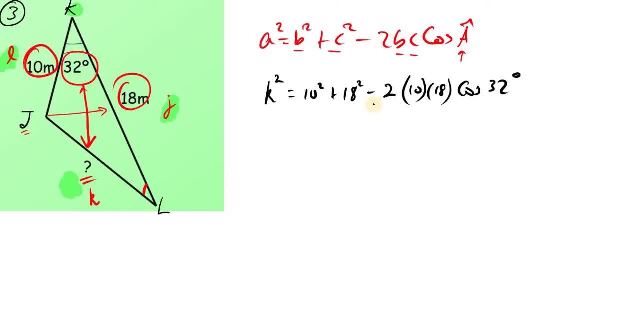 of the angle that's formed between them, which is 32 degrees. And then we say K squared is equal to, and we can plug this entire thing in our calculator. Your calculator should be able to do all of this one time. So I'm going to put 10 squared plus 18 squared. 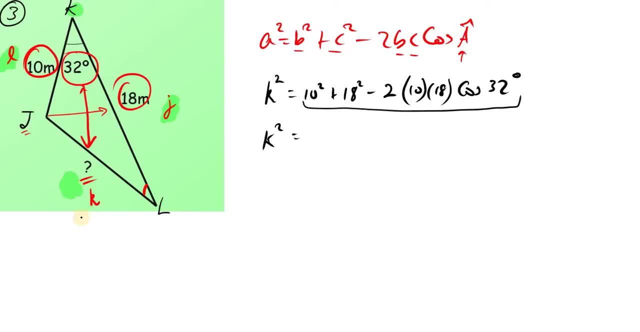 Okay, Okay, Okay, Okay. Okay, now, assuming your calculator can't do that, I'm gonna just work out them in bits. there's not everybody's calculator can actually work these out one time. so, doing them in bits, I'll work out this portion. then I'll work out this portion. 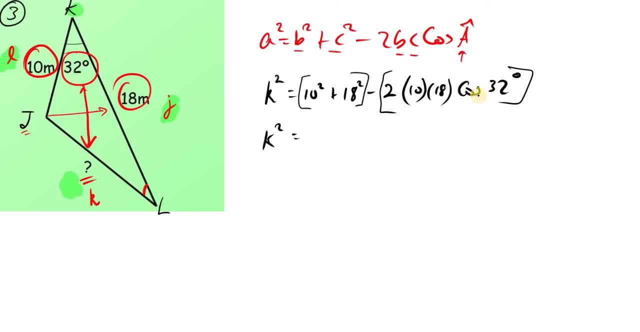 this portion, here everything is multiplying, so you have to work out all of that first. so for this portion here, the additional portion, that's 424, minus this expression, here our term. so we say 2 times 10 times, 18 times cosine of 32, close bracket and that gives me a minus three, oh, five point two, nine, seven, three. 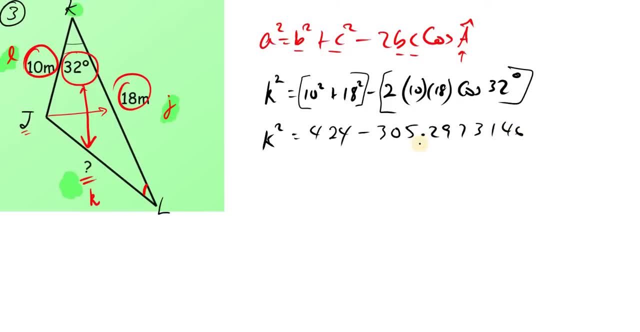 one, four, six, etc. but I want three decimal places. all right, so three oh five, point two, nine, seven. I'm gonna chop all of this off, since this is since the first of those we're trying to do, is we're trying to do, is we're trying to do. 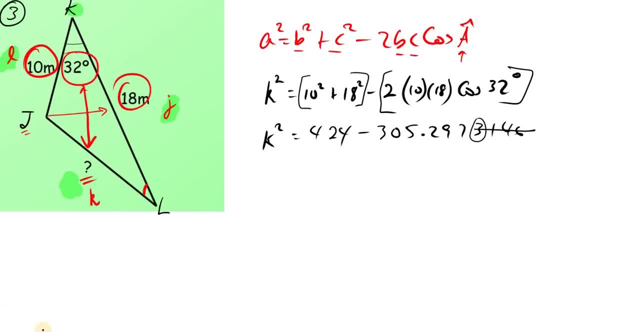 one more time. so we robbed an office. less than five. I'll keep my seven as seven, so all of these will go, and so also key squared is equal to- so I'm gonna work that out- 424 minus 305, 0.2 97, and I'll give me one one eight point. 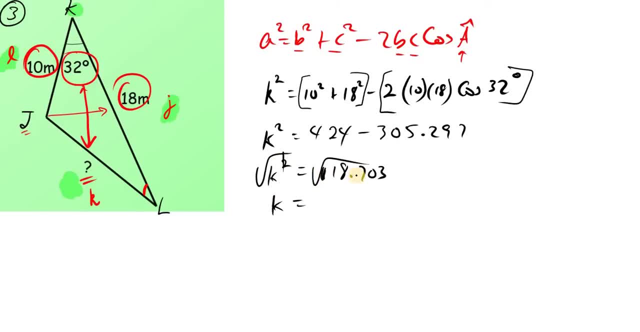 seventy three. so K is equal to norm to remove this clear root. so I square both square root both sides. what's the scary of? sorry y'all, we don't have enough time because of the criteria and I can'tparent 118.703.. So I'll press the square root button. 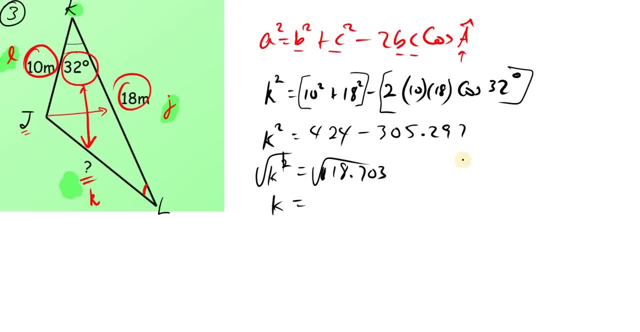 then I'll press the answer key, because this figure here is toward the answer key. In the answer key I'll have the 118.703.. So when I press the square root button on my calculator and then I click on answer, what's in the answer is really this: 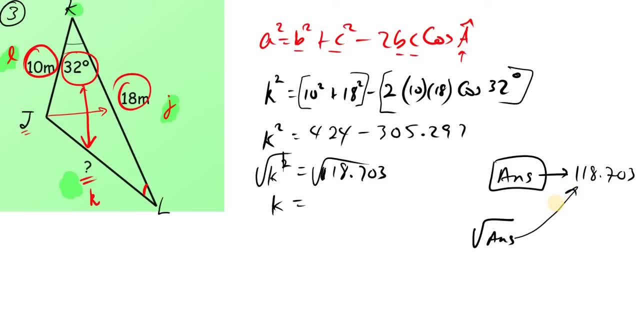 So I can just press the answer key after I press square root and then equal, and then I'll get 10.895, three decimal places, but I want three significant figures in my final answer. so that's 1, that's 0 and the 8 here. But checking the next digit, 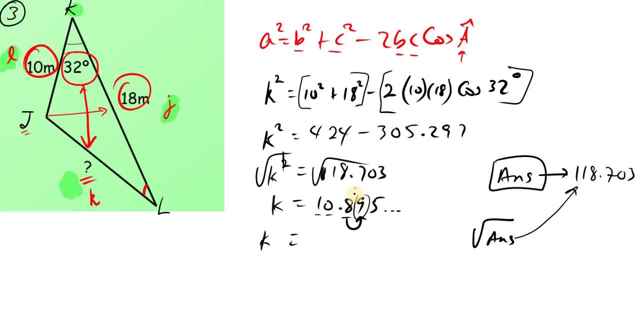 it's in the category of 5 or more. This digit I'm going to chop off. it's in the category of 5 or more, so I'm going to add 1.. So we're going to get 10.9.. And since we did it with meters in this case, 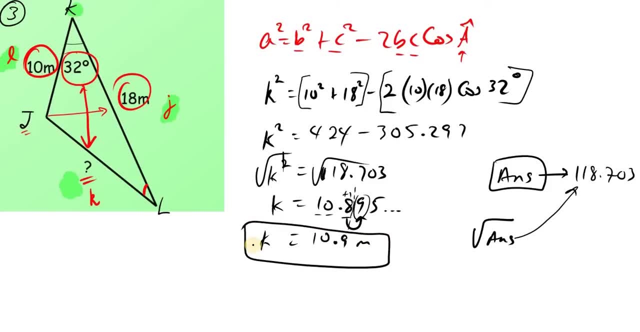 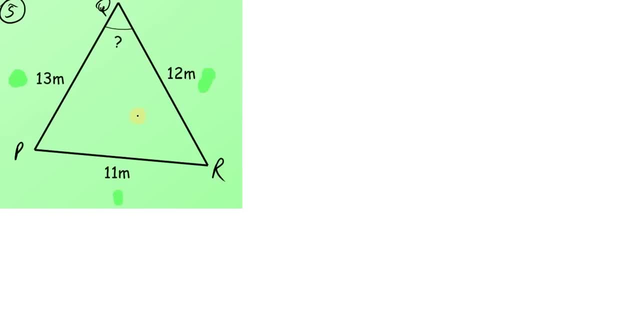 then my answer is in meters. Okay, next, Let's look at this one. Am I going to use sine rule or cosine rule? Now, what I have here is the angle. What I have here is an angle that I need to find. 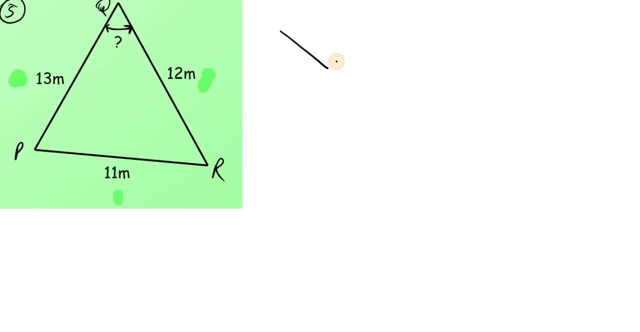 But remember, for the sine rule we need what Known, known, unknown, unknown. The unknown could be anywhere that k is, but everything else has to be known. So we must have three. As long as we have three knowns and one unknown, then we use the sine rule. 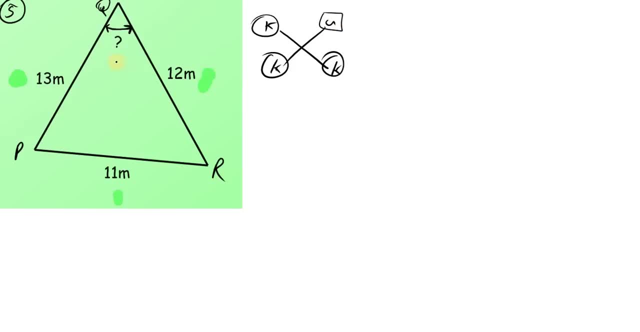 Is that the case here? Well, let's look, If I draw a line here, what I have here is I'll have one unknown from this end and one known. So the angle is unknown, the side is known, But the fact that we don't have any more angles we cannot. 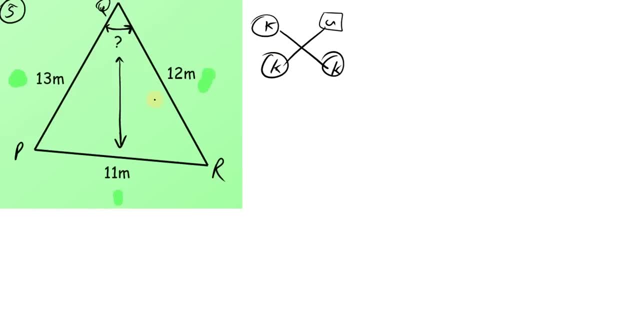 find a known and known. Remember you know, we must have side to angle. This is the angle, then this is the side, This is the side and this is the angle. So this is unknown and this is known. So we cannot find another pair, a full pair, to give us a sine, to use a sine rule. 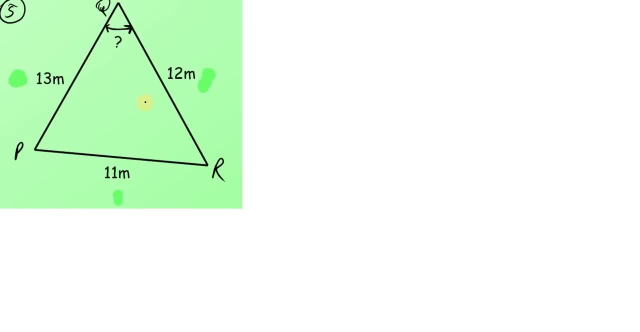 Can we use a cosine rule though? Yes, You said. yes, you're correct. Cosine rule is when we deal with all three sides and included angle. For the three sides one could be unknown, which means that the included angle must be known. 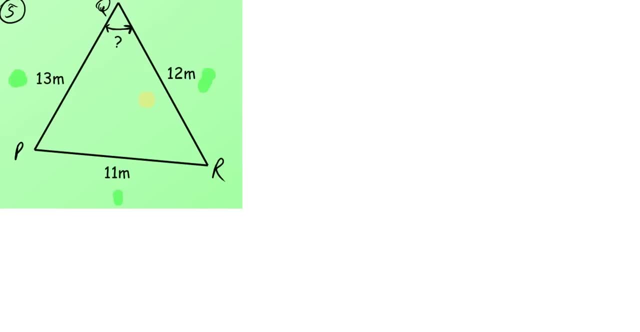 If one of the sides is unknown, If all three sides are known, then the included angle must be unknown Again. that's why we use the cosine rule. So the cosine rule- three sides must be given if you want to find an angle. 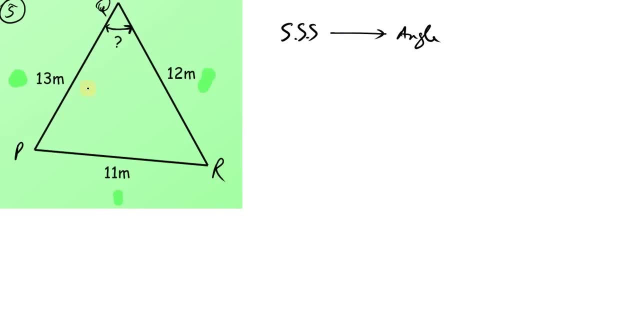 Three sides must be given if you want to find an angle. So we have three sides given and we want to find an angle. So, given what are we trying to find? Sometimes you may have to find A side, so that means you must be given what. 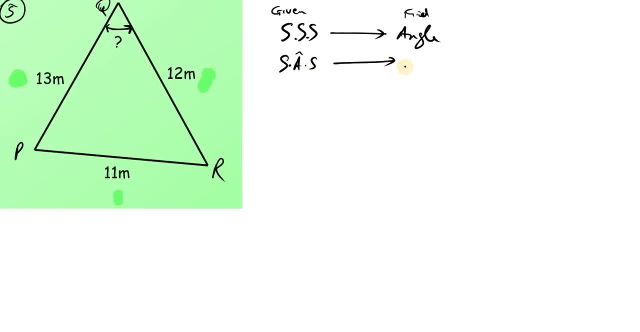 Two sides and the included angle in between those two sides when you want to find the other side. So we're looking at this case, All three sides given an angle, But we need to identify in the formula what The two sides that form the included angle. 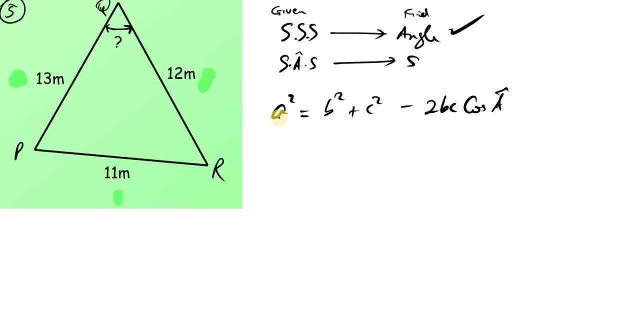 So, if you look at this, we have A facing angle, A Right, so, and B and C are what The two sides that form the included angle? Now, which two sides form the included angle here? What's the included angle? The included angle is what we're trying to find. 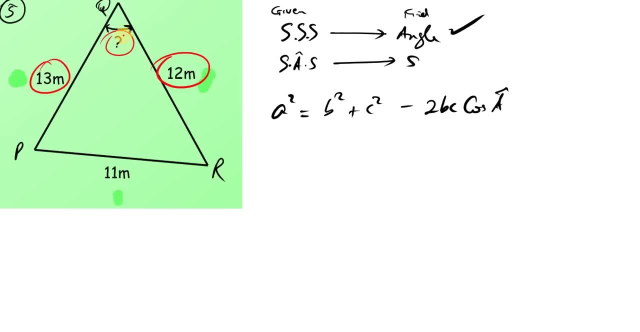 So we have these two sides that form them, that form this included angle here. So this would be my B and my C in terms of the formula, The two sides that form angle A, And the side A here is the one that faces the angle. 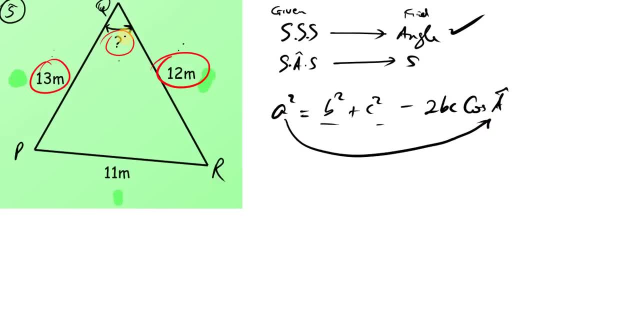 So notice A facing angle A. So angle A is here in this, which we're given as Q in this case, and side A is here. But notice that we're trying to find actually the angle, isn't it? We're actually trying to find this angle. 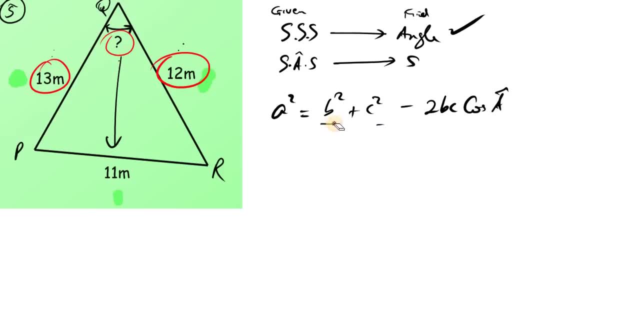 So here's the thing, Here's what we could do to make our lives easier. To make our lives easier, we can rearrange this formula so that A is in the is the subject or close to being the subject. Notice that everything here is being. 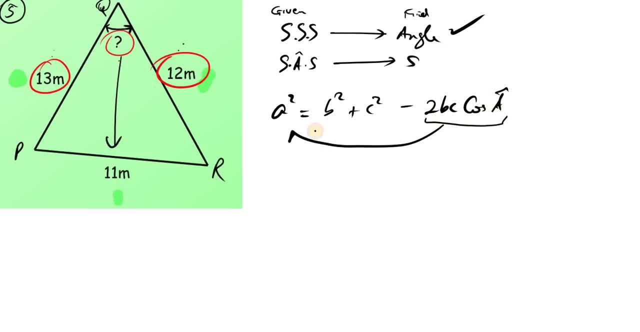 is multiplying correct. So what we can do, we can transpose this term here: negative. two B- C equals cos A. We can transpose that term and then transpose the A squared. So what we're gonna have is this portion becoming positive after transposing over the equal sign as positive: two B- C, cos A. 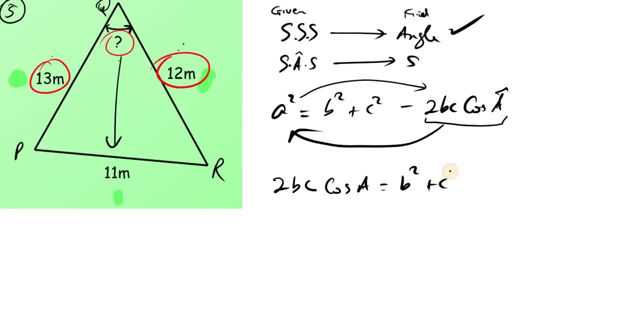 And transposing A squared over, we'll have the B squared plus C squared and A squared, becoming negative A squared. Okay, And even to make this easier too, we can get rid of the two B C. Two B C is actually doing what? 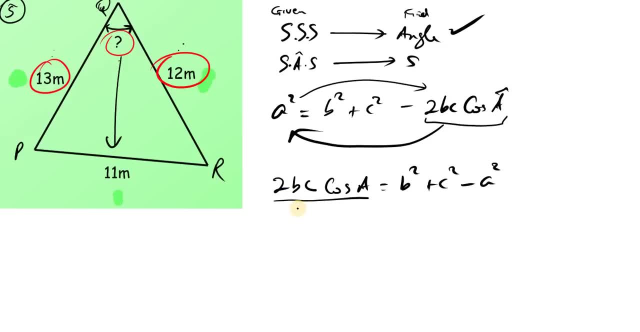 Multiplying cos A, so we can get rid of this: two B C. Let's do that quickly. Two B C, right, Two's constant, two B constant, B C, constant C. And we divide over here as well by two B C. 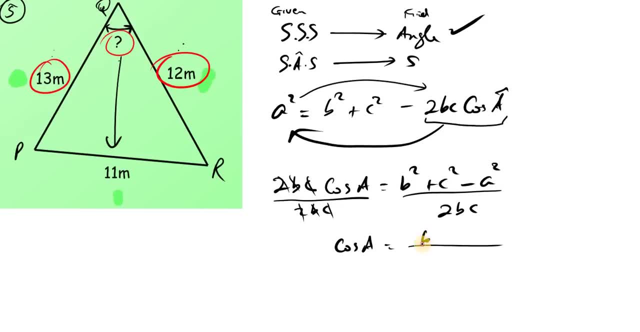 So now we have: cos A equals this B squared plus C, squared minus A squared over two B, C. So this little formula here will make it easy for us to work out the solution. So let's do it here. So cos of angle A is equal to what? 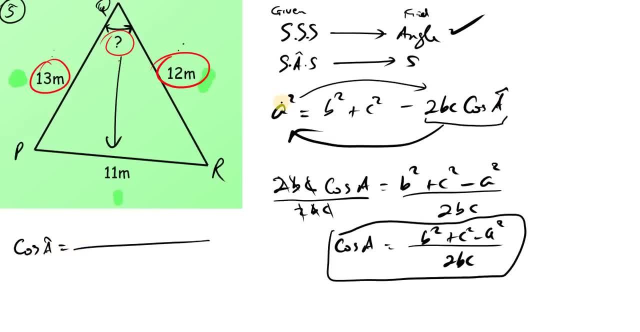 In this case, angle A again, which is the side that faces B, is angle that is trapped or formed by B and C And forming by these two sides is this angle. So it's really angle Q in this case. So angle A is our angle Q in that sense. 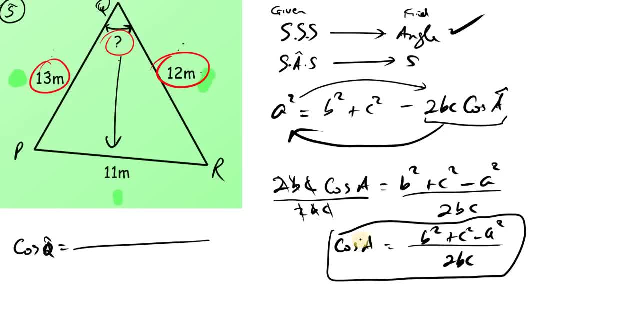 What two sides that form angle Q. It's 30.. It's 13 and 12.. What do we do with them? We square them and add them according to this little formula here, right? So we're going to square 13,, square 12,. 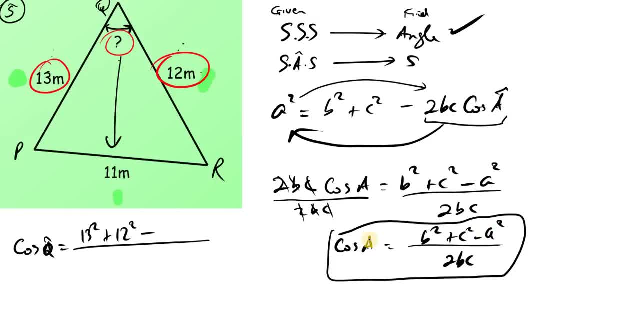 then subtract the side opposite, angle A, In this case angle Q. So the side opposite is this side here, 11 squared over two times the B and the C, So two times the 13 and the 12.. Okay, so this might make it a little easier, right. 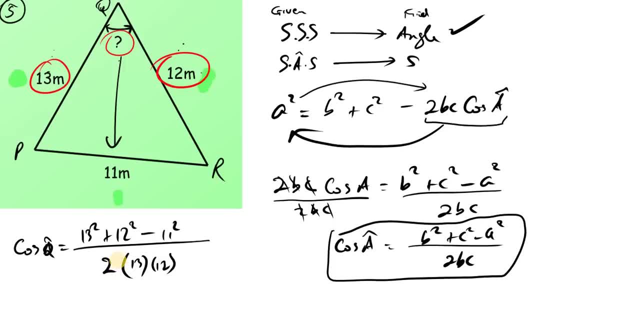 So we're going to do this. So we're going to do this, So we can work out the top: 13 squared plus 12 squared minus 11 squared equal what? 192.. And two times 13 times 12 is equal to 312.. 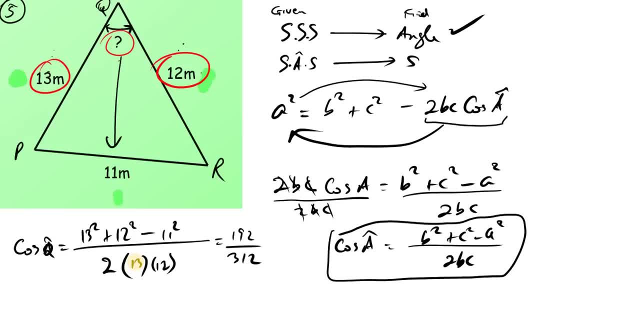 And if I work this out, let's put 192 back in our calculator divided by 312.. The R is important, so make sure you write the 192.. 192 first, then division sign, then 312.. And then you're going to get. now I'll get 8 over 13.. 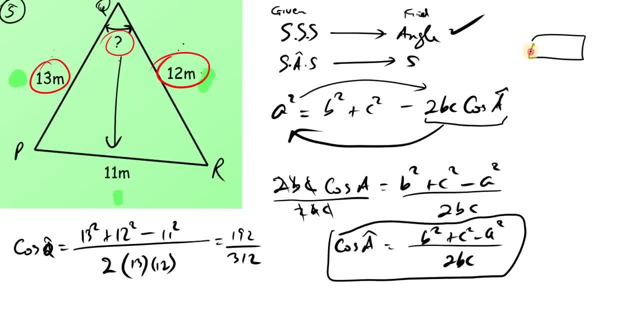 So you want to press this button. Press this button that you're seeing, In case you get a fraction. you want to press this button, Standard to decimal Right. press that button and you should see 0.6153, etc. But since the next digit is 3, then I'll leave this 5 as it is. 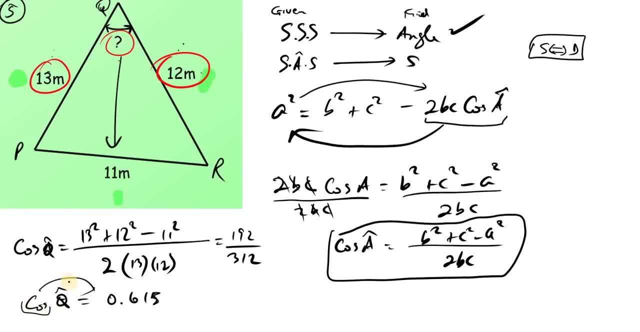 Okay, and I'm going to transpose just the Q I want. I'm going to transpose to the other side, Because I'm transposing the cosine, then leaving the Q, then the cos by itself goes over as cos inverse, Since I'm moving cos over by itself. 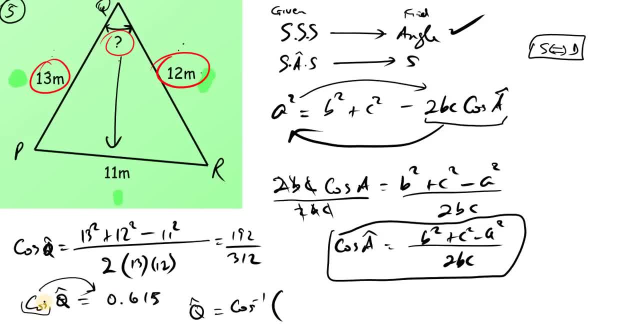 I'm not carrying cos Q over the equal sign, I'm just carrying the cos alone. So that's cos inverse of 0.715, which means that angle Q shift cos inverse 1 to the right. I'm going to just press the answer that I had before and I'll get 52.0.. 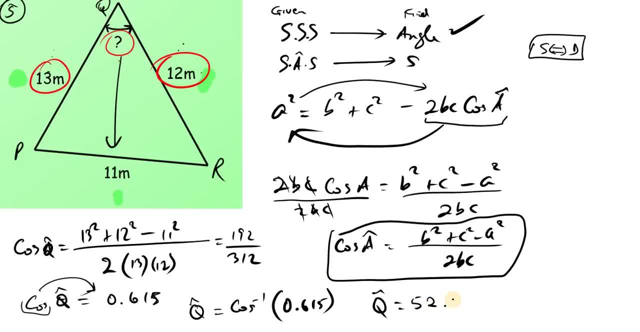 I've got 0 as a 2 there, so I can just leave that as 52.0 degrees. All right, now I just use answer. that's so that I really have the long answer instead of this. So if I actually do the shift cos inverse of 0.615, let's see exactly what would I get. 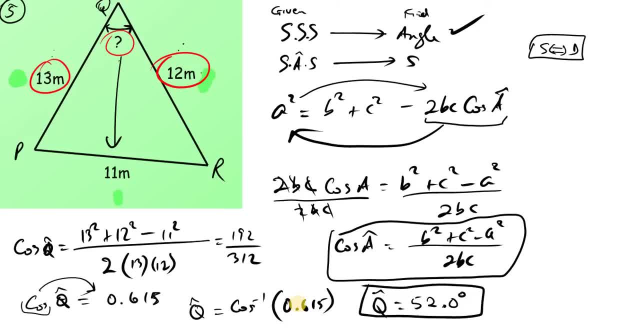 for that. Oh, I'll get 52.04.. So because a 4 comes after the 0, we'll still maintain it as 0, so that still works, Okay. so let's see if we have another one. We have an angle to find. 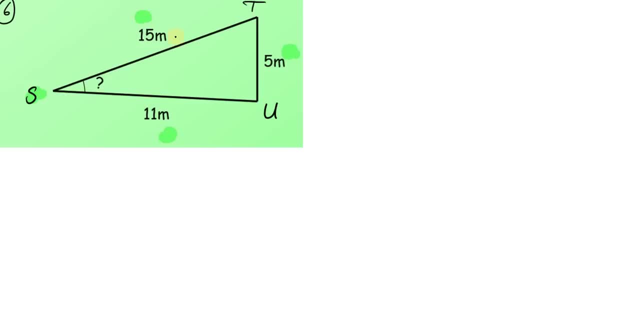 Okay, can we use the sine rule? No, because we're given what? Three sides and the included angle. So now that we have the formula, remember it's the angle that we're trying to find, But we can replace Opposite angle. S is little s. 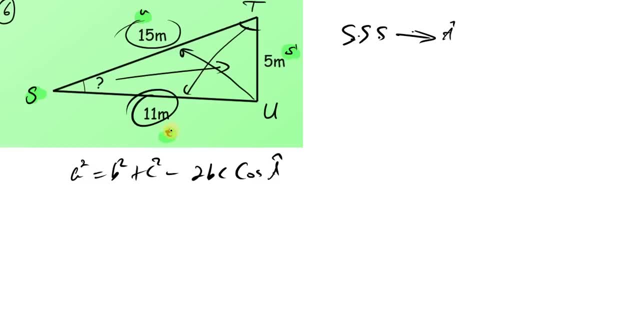 Opposite angle S is little s. Opposite angle T is little t. side T. Opposite angle U is little u, So A in this case is facing the included angle A, So this is the included angle, since we have these two sides that form the included angle. 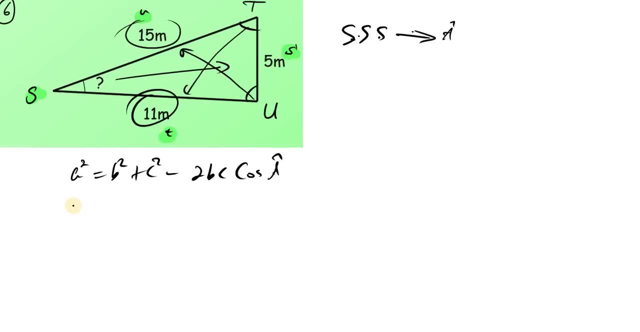 So opposite included, angle is 5, all right, So that's 5 squared is equal to B, and C represent the two sides that form the angle. so that's 15 squared plus 11 squared. Does it matter? we have 15 first, or 11?? 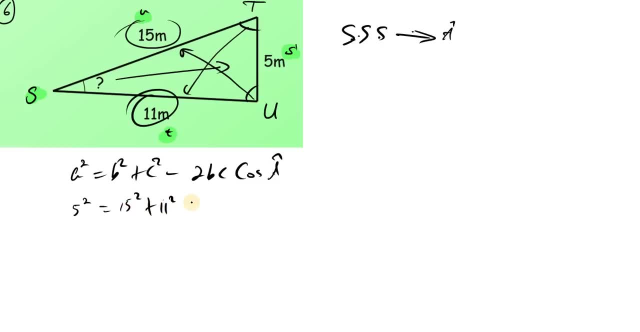 No, It doesn't matter if we have 11 first or 15 first, because the order which you add doesn't matter, right? So that's 2 times 15 times 11, cosine of the angle that's included between the two given. 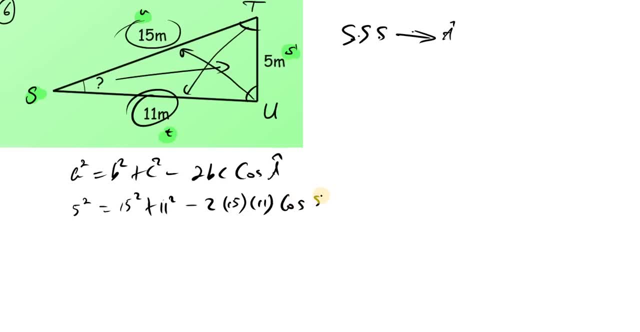 sides, So the angle included is really angle S, but we do not know its measure for now. right, Do not know the measure for now. So what I'm going to do, though? remember what we did last time? all right, I'm going to transfer this 5 squared over, all right? 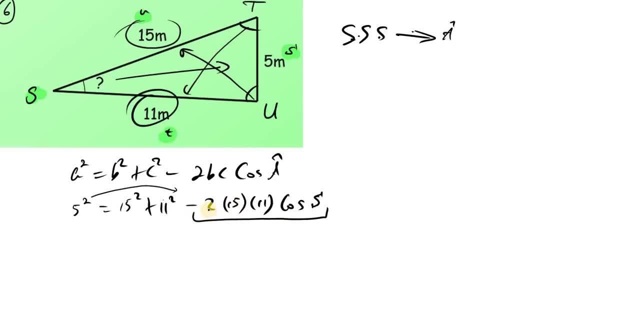 And then see this angle, This product here, because everything is multiplying here. This is really one term. We can't work out this portion 2 times 15 times 11 and subtract it from the result of 15 squared and 11.. 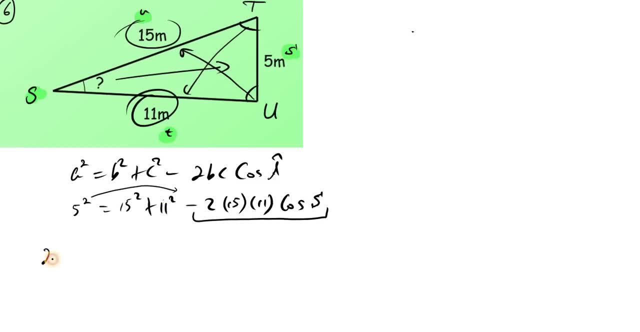 But I'll say I'm going to carry this across so it become positive 2 times 15 times 11, cos of S, angle S, that is, I'm going to transpose the 5 squared over, So that's 15 squared plus 11 squared minus 5 squared. 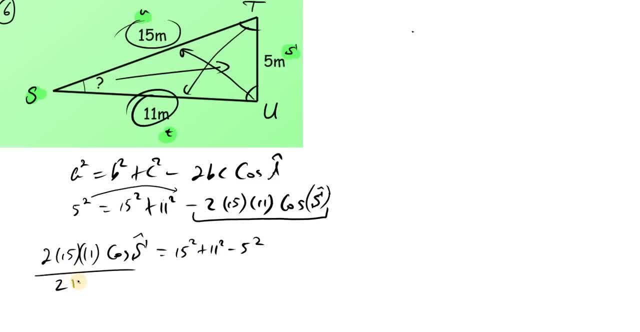 Then I can get rid of this 2 times 15, right, 2 times 15 times 11, I can get rid of those Divide over here as well, by 2 times 15 times 11.. So what I have so far is that what cos of angle S is equal to 15 squared plus 11 squared? 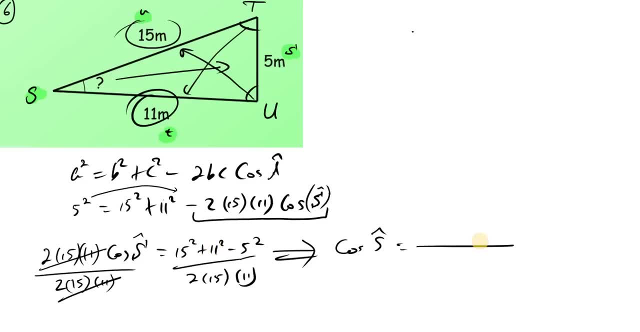 minus 5 squared. Let's write that out, All right: 15 squared plus 11 squared minus 5 squared, That's going to be 321, and then below we have 2 times 15 times 11.. That's 330.. 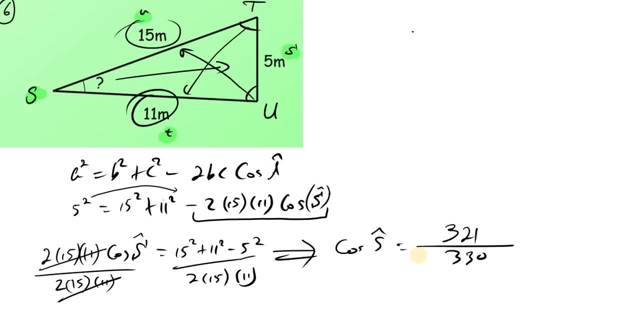 So we're going to divide. Make sure you divide. put in the top number in the calculator first, So 321.. Then you press division 330.. Simplify that to 107 over 110. But I want the decimal, so I'm going to press the SD button. 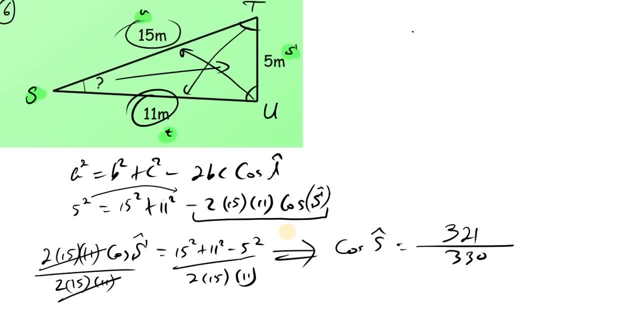 What do I get? OK, So let's press it twice So you can see that is 0.972727XS. So my calculator I have is 0.972 and a dash over 72. What it means here that after 0.972,, after 72, you have another 72.. 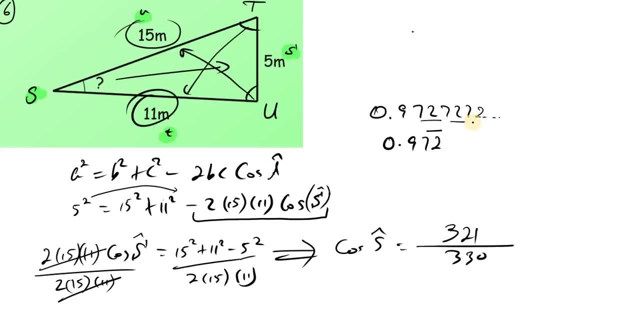 I keep on having 0.972.. I keep on having 0.972.. I keep on having 0.972.. Then I keep on having 0.872 again, and it will continue on forever. So what we can do, therefore, is press the SD button again, and it will now give us this: 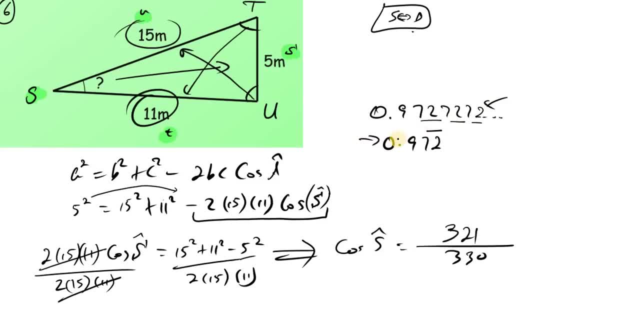 one instead of actually this. So we can clearly see now that, OK, if we want three decimal places, then it's going to be what 0.97 do? that's two decimal places. Now to put the third decimal place, we need to ask ourselves: 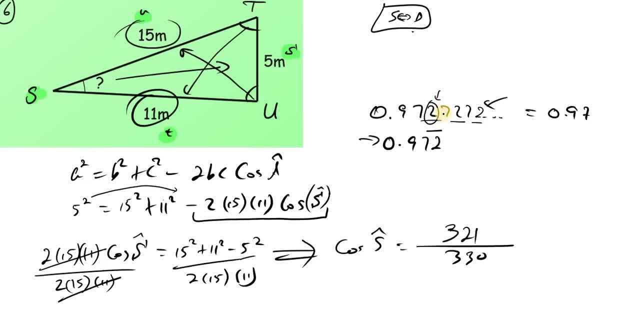 Should we add one to this guy here or maintain it? well, check the next digit. it's actually what seven and seven falls in the category of five or more. so we're gonna add one, two and get three. so it's zero point. nine, seven, three. so in fact, you know what you could have done. 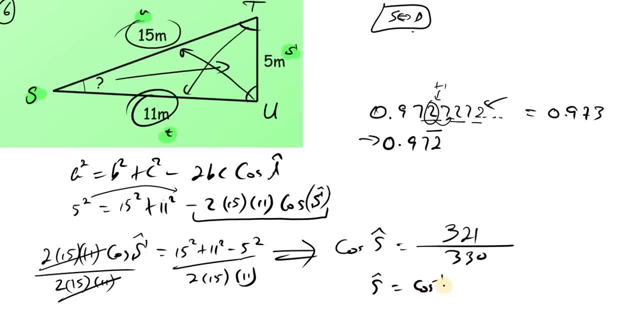 though gonna put s angle. s is equal to cos inverse and just leave this in your calculator: 321 divided by 330. all right, rather than going through this whole drama there of trying to do all of that and then you. then you go, shift cos inverse and you put in your values: okay, so you can either put this in there as: 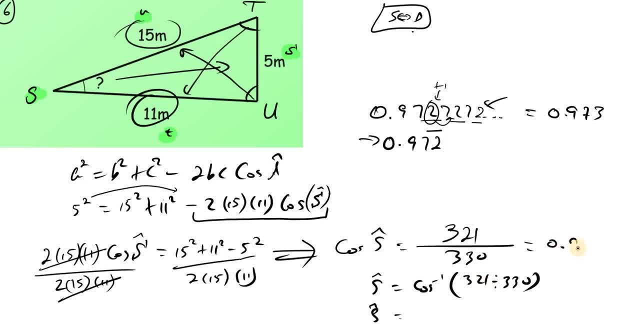 it's given there. if you actually round this off to zero point nine seven three, then you can press c cos inverse of zero point nine seven three, and then let me just put the last one, zero point nine seven three, close bracket, and you get your answer to be: